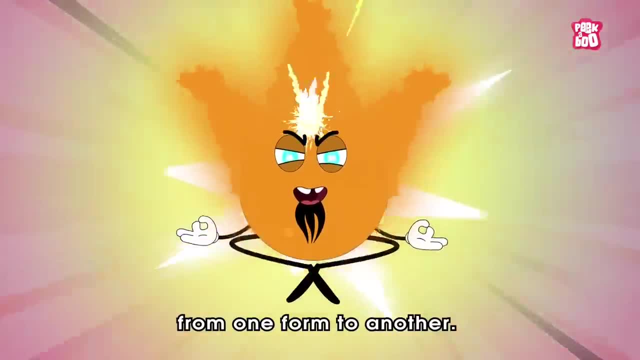 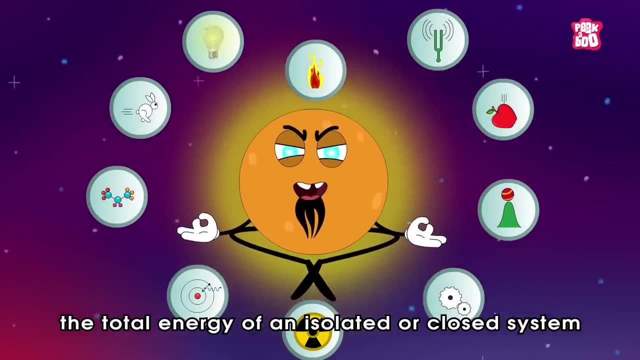 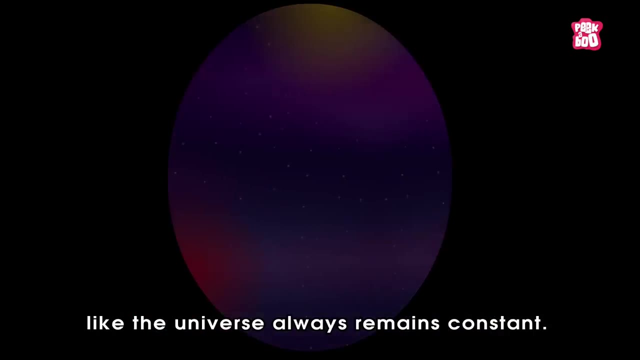 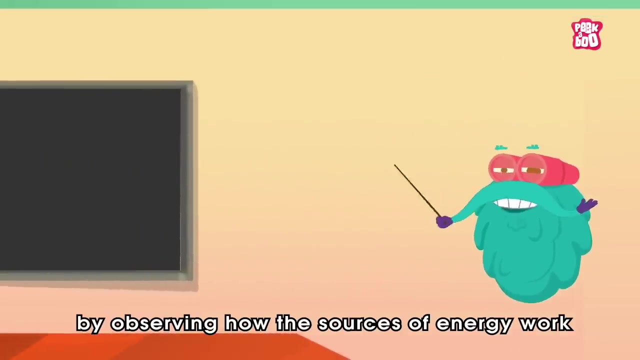 But it may be transformed from one form to another And if you take all forms of energy into account, the total energy of an isolated or closed system, like the universe, always remains constant. How We can learn more about it? by observing how the sources of energy work. 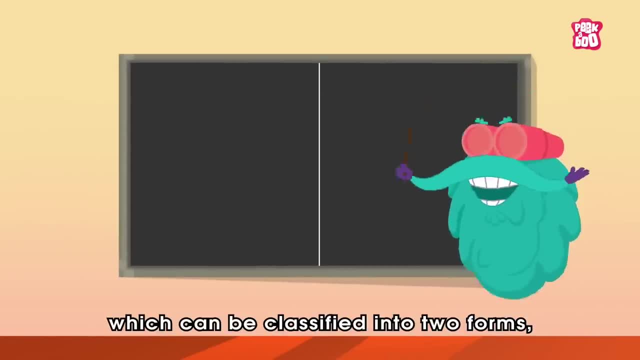 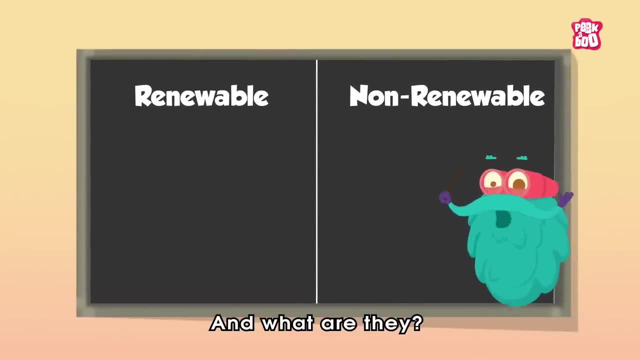 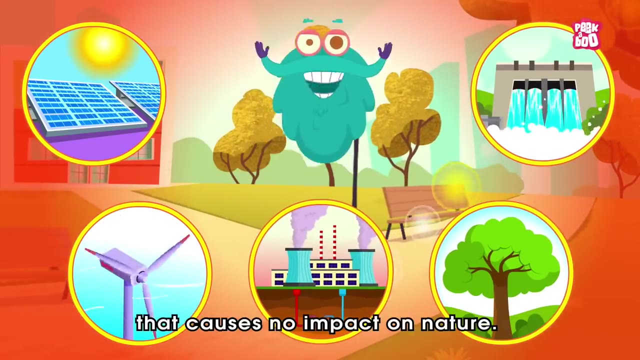 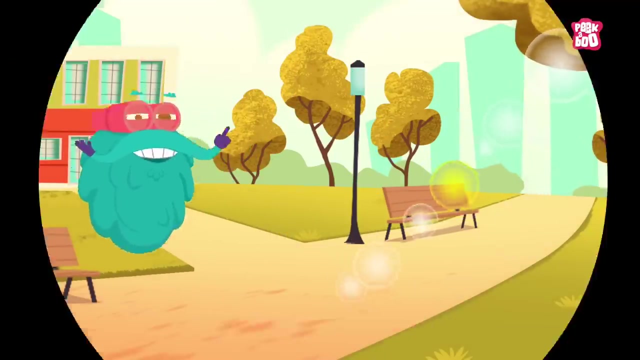 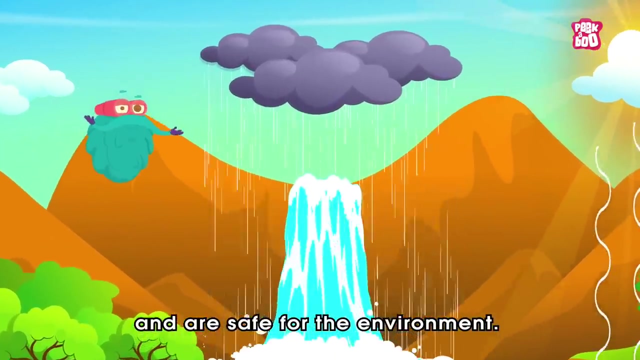 which can be classified into two forms: Renewable and non-renewable sources of energy. And what are they? Renewable source is a natural resource that causes no impact on nature. They are available in abundance in nature and are sustainable. These resources of energy can be naturally refilled and are safe for the environment. 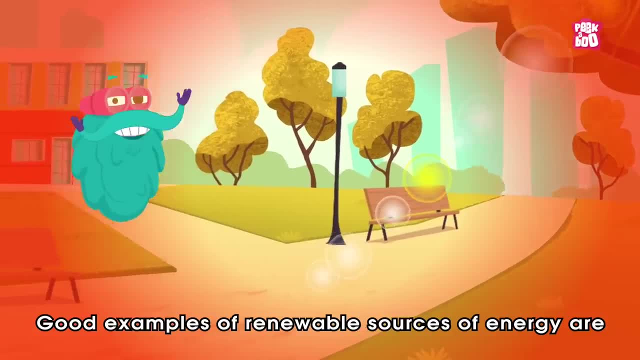 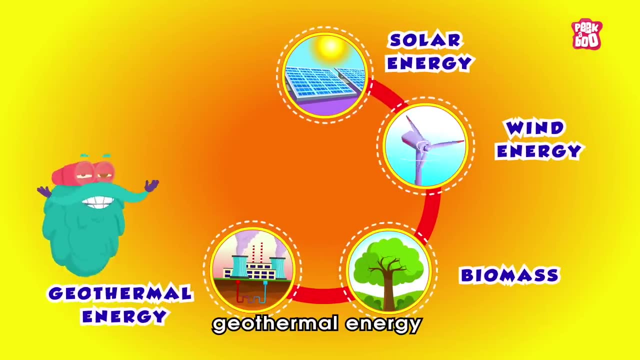 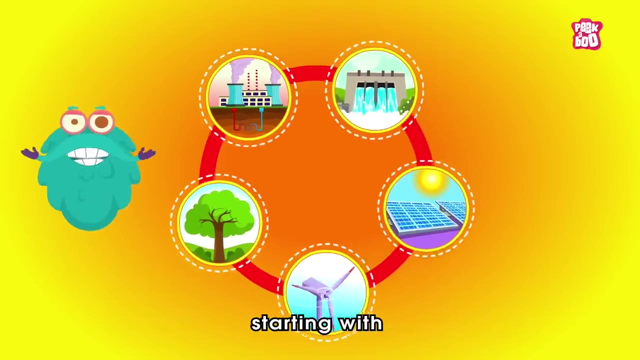 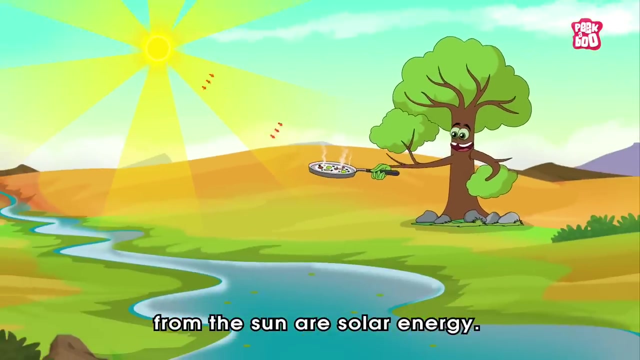 Good examples of renewable sources of energy are solar energy, wind energy, biomass, geothermal energy and hydropower energy. So let us look at them one by one, starting with solar energy. The heat and light we receive from the sun are solar energy. 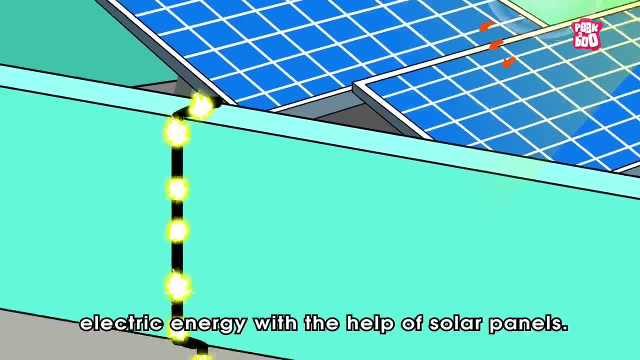 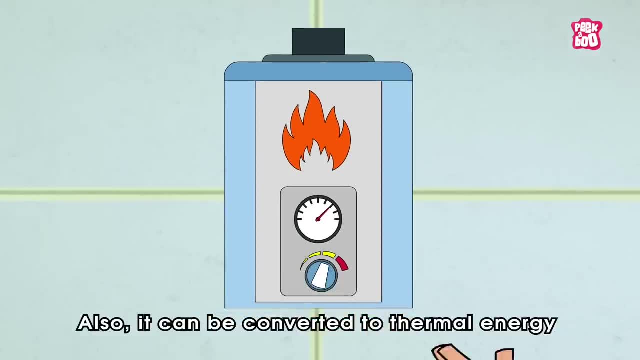 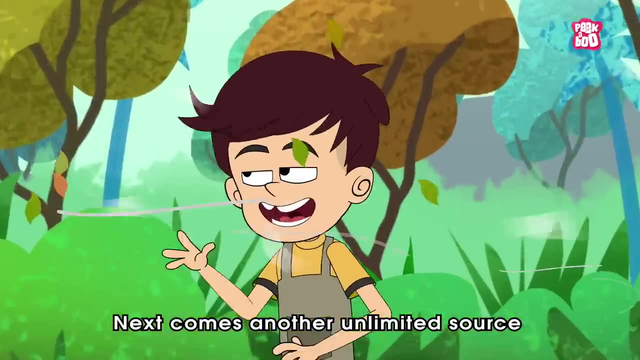 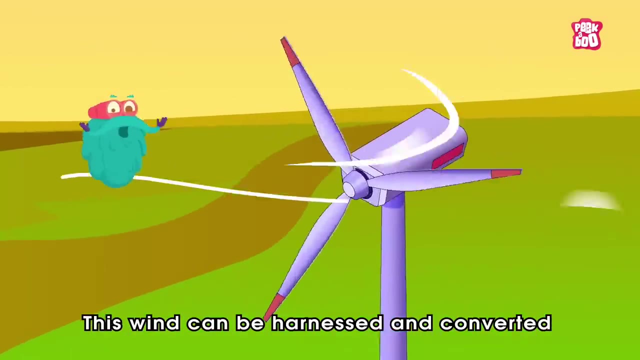 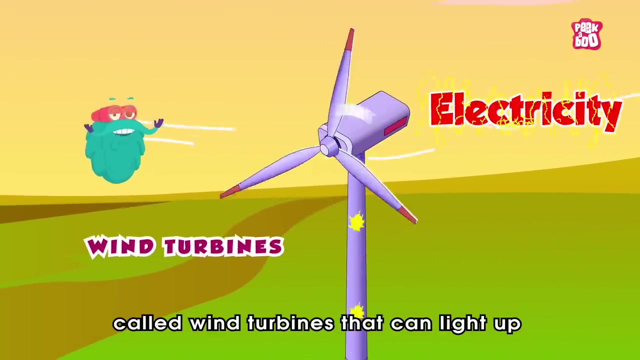 This energy is then converted into electric energy with the help of solar panels. Also, it can be converted to thermal energy to heat our homes or water. Next comes another unlimited source called wind energy, which is produced through the wind. This wind can be harnessed and converted into electricity using man-made structures called wind turbines. 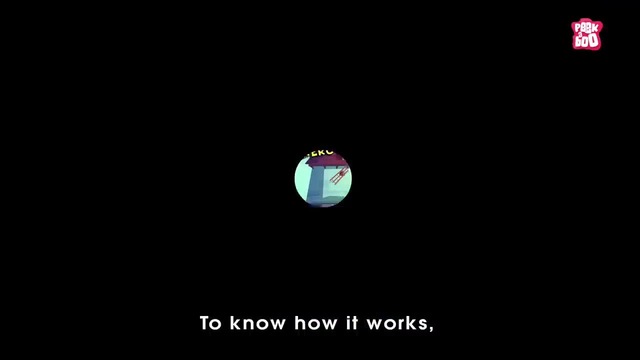 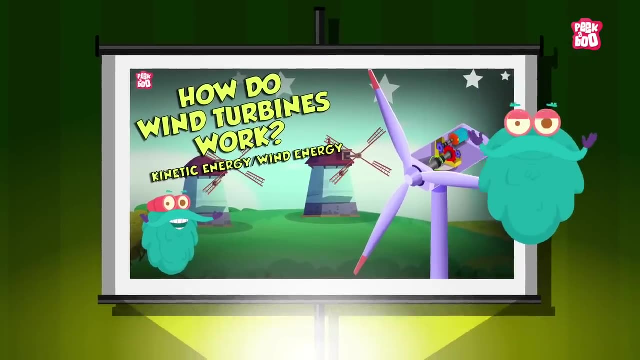 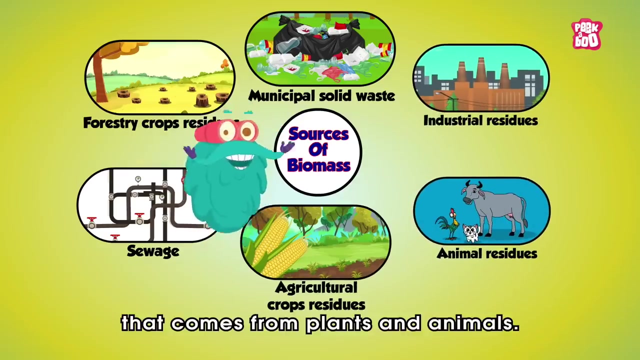 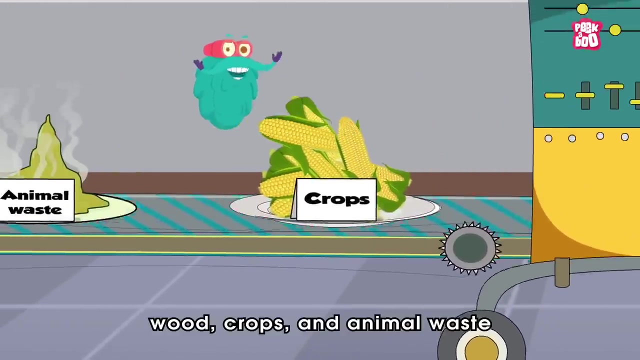 that can light up our houses and schools. To know how it works, please check out our video. How do wind turbines work afterwards? Now let us look into biomass, which is renewable organic matter that comes from plants and animals. Examples of biomass include wood crops and animal waste that can be turned into fuel.